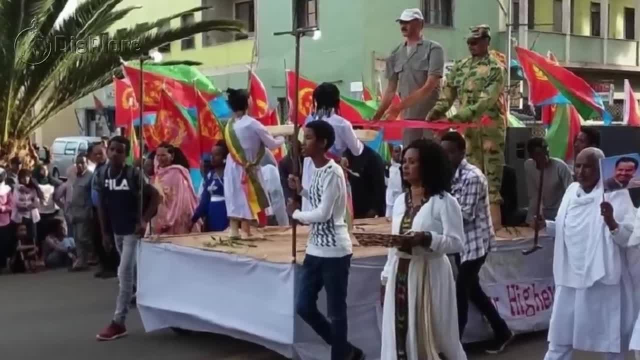 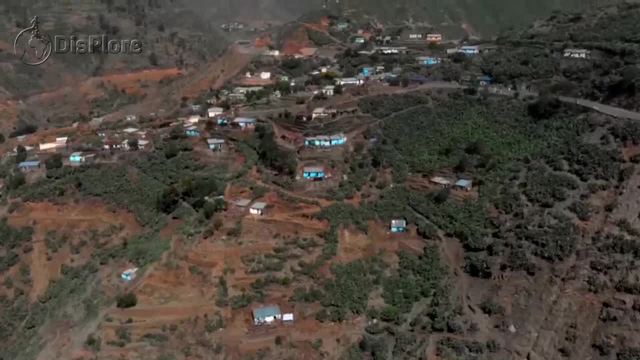 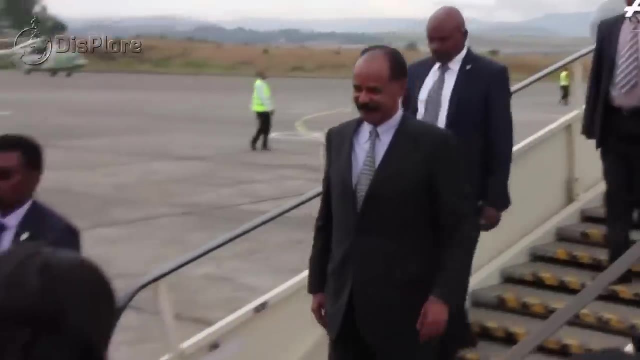 World War. Eritrea got its independence on May 24, 1991 after a tussle with Ethiopia. Eritrea is a country with rich history and an old civilization dating back to several thousand years ago. The capital city of Eritrea is Asmara and the current president of the country is Isaiah Afwerke- If you're new here. 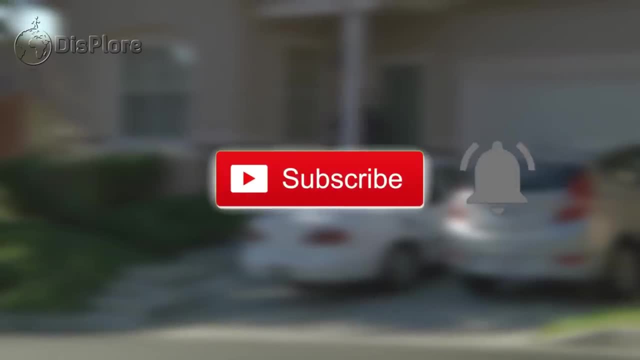 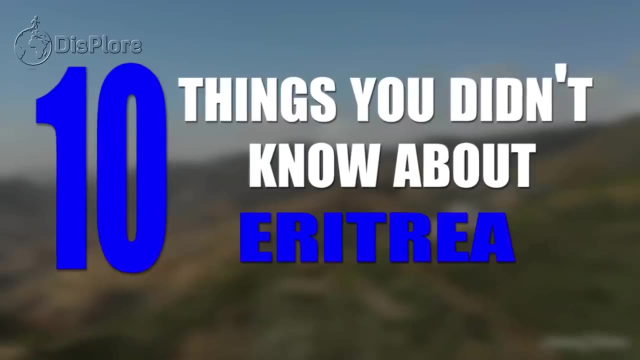 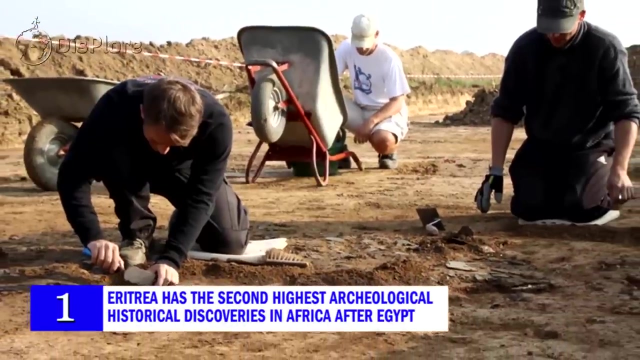 welcome. Be sure to subscribe and turn on notifications so you don't miss any of our videos. Eritrea got its independence from Ethiopia in 1991.. And with that said, here are 10 facts about Eritrea. 1. Eritrea has the second-highest archaeological historical discoveries in Africa after Egypt. 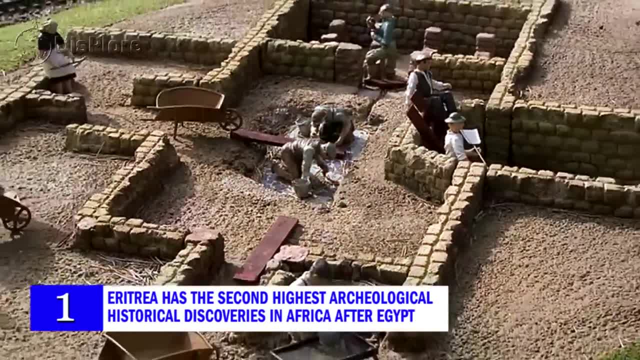 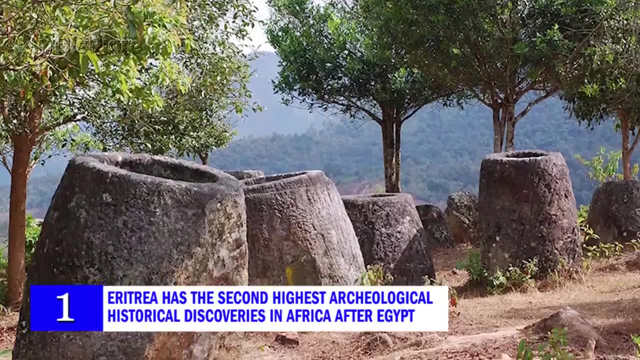 Eritrea is an ancient civilization dating back to thousands of years ago. It is a land that had been inhabited by early humans for long. It has one of the ancient human habitats, evidenced by the high number of archaeological sites that reach almost 80,000.. These numerous 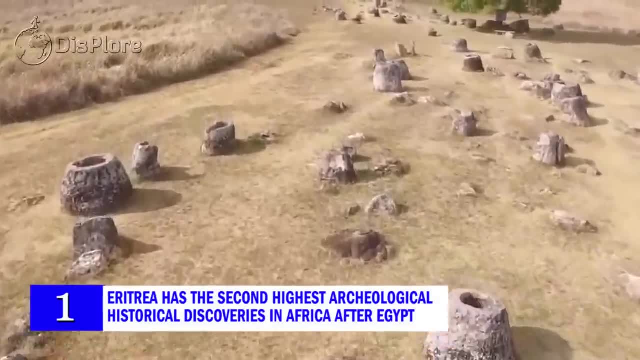 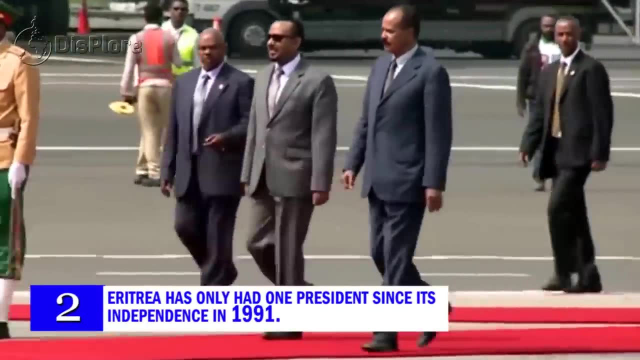 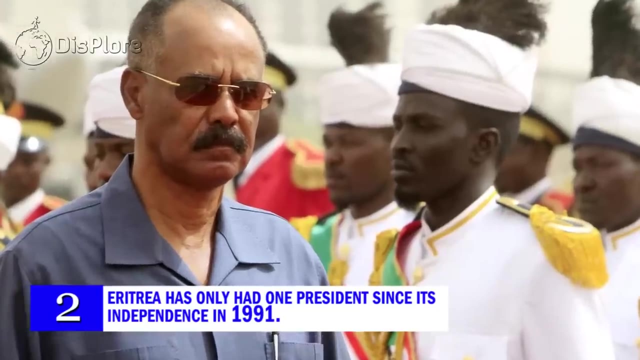 archaeological sites are proof of early human habitation. 2. Eritrea has only had one president since its independence in 1991.. Since Eritrea gained independence from Ethiopia, there's hardly been elections, despite the first one having been scheduled in 1997, after the adoption of the constitution that declared: 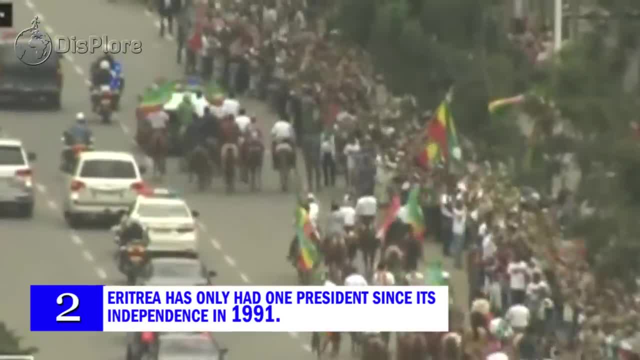 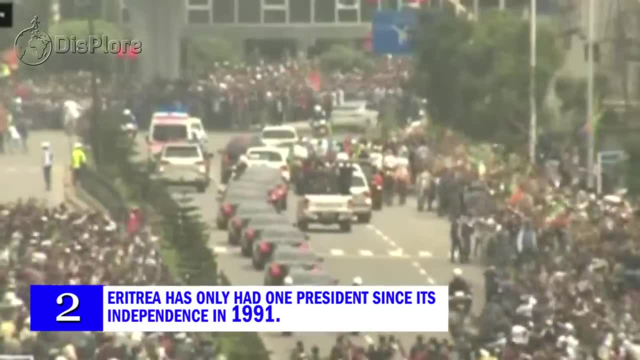 Eritrea as a multi-party democracy. The current president of Eritrea is Isaiah Afwerke, a position he's been occupying since the independence of the country in 1990.. 2. Eritrea has the second-highest archaeological sites, dating back to the physicists in the 19th century. This is because: 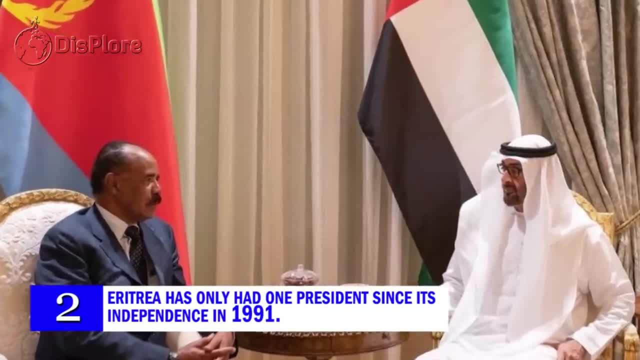 Eritrea is the second-highest archaeological site in Africa. 3. Eritrea has its own culture of coffee. celebration War with Ethiopia was used as justification for postponing the first scheduled elections. Afterwards. there have been mountains of excuses not to hold another one to date. 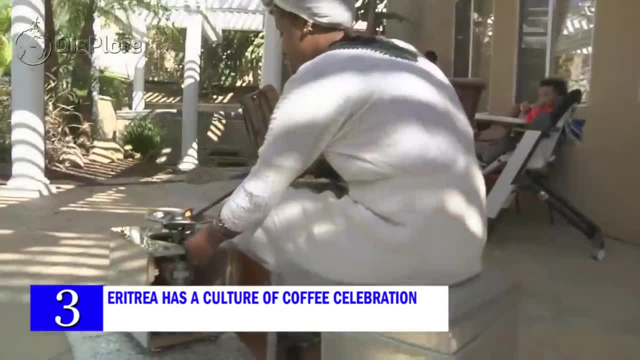 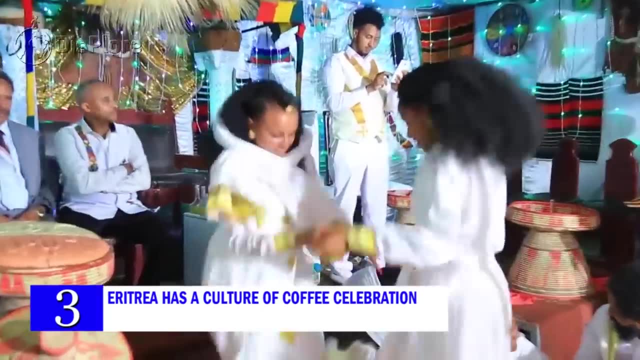 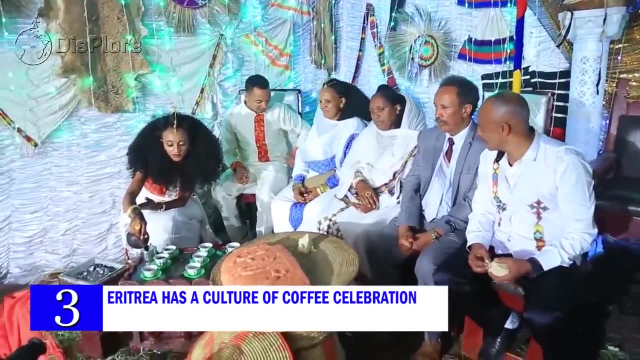 3. Eritrea has a culture of coffee celebration. One of the most recognizable parts of Eritrean culture is the coffee ceremony. During the coffee ceremony, there are traditions that are upheld. The coffee is served in three rounds. The first round is called awel in Tigrinya, meaning first. The second round is called 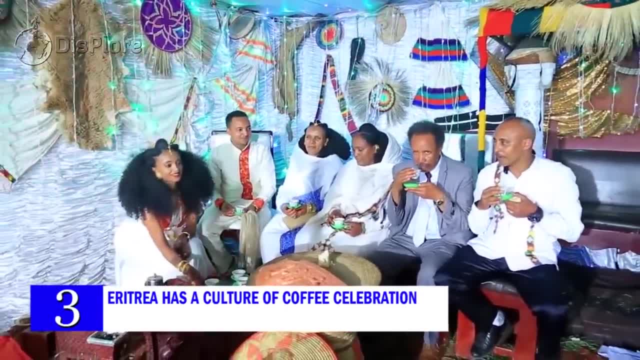 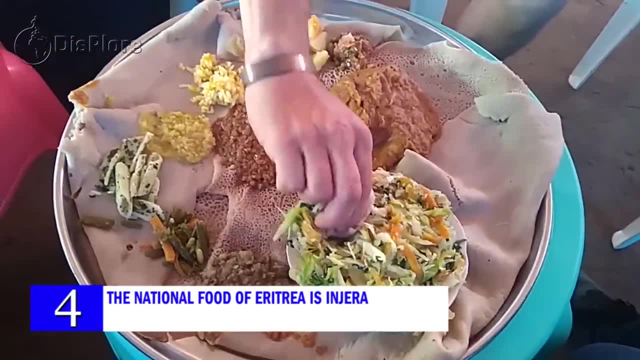 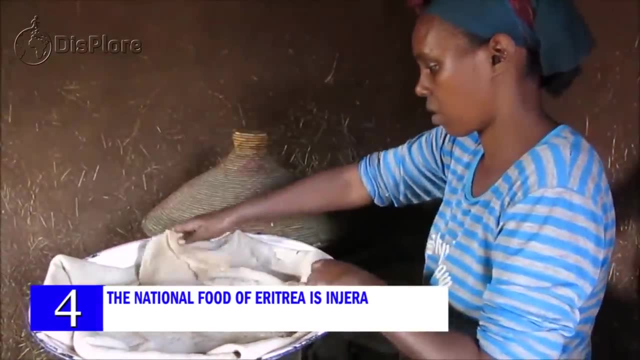 Kalei, meaning second, and the third round is called Bereka, meaning to be blessed. Number 4: The national food of Eritrea is injera. A typical traditional Eritrean dish consists of injera accompanied by a spicy stew which frequently includes beef, chicken, lamb or fish. 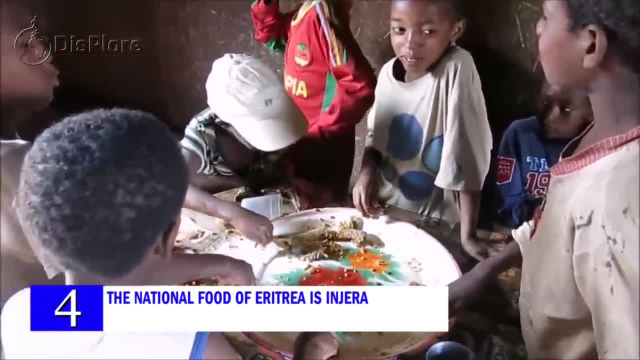 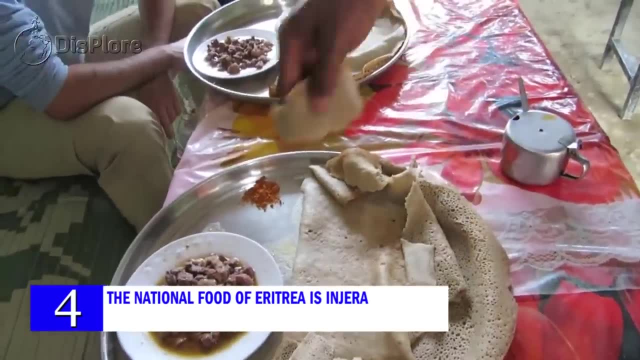 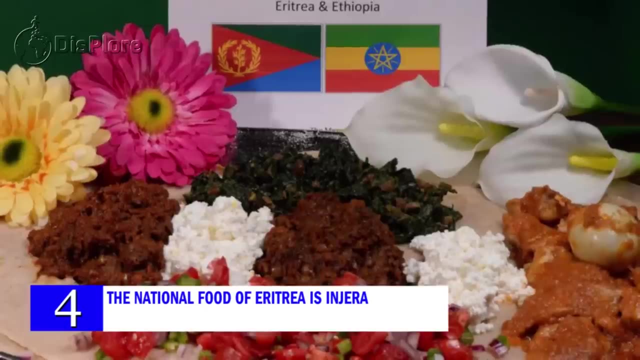 The overall Eritrean cuisine strongly resembles those of neighboring Ethiopia, Though Eritrean cooking tends to feature more seafood than Ethiopian cuisine. on account of their coastal location, Eritrean dishes are also frequently lighter in texture than Ethiopian meals, But they likewise tend to employ less seasoned butter and spices and more tomatoes, as in 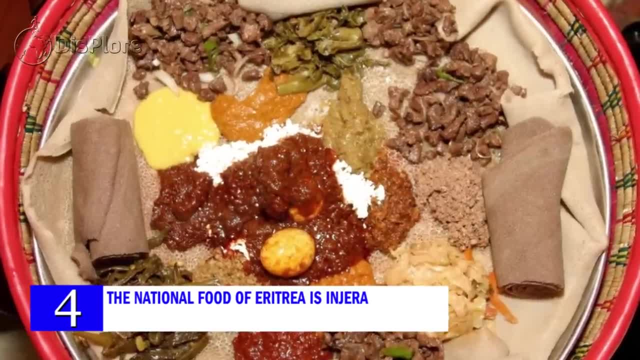 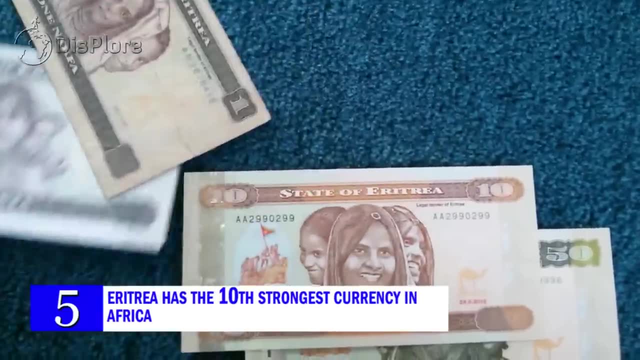 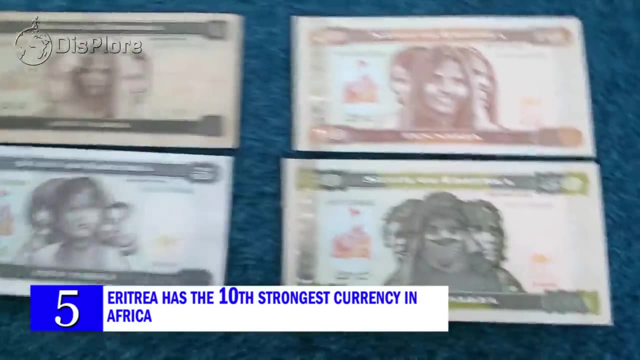 the Tebidoro delicacy. There are several very popular dishes in Eritrea, but the national food of the country is injera. Number 5: Eritrea has the 10th strongest currency in Africa, Though Eritrea is one of the youngest countries in Africa, having gained independence in 1991,. 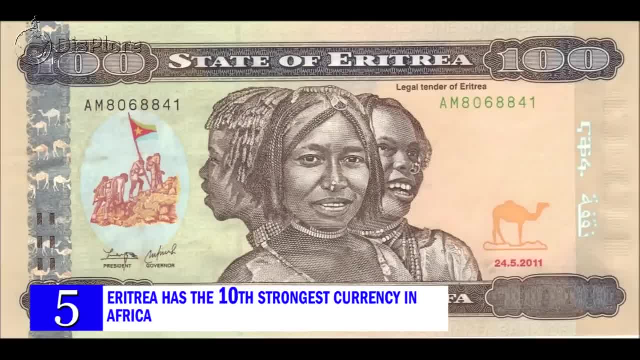 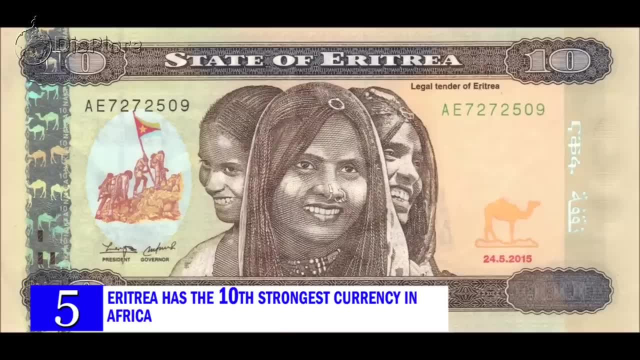 the country has one of the strongest currencies in Africa. To better understand the strength of the Eritrean currency called Nekfa, let's put it against one of the most popular currencies in the world, American dollar. One US dollar is equivalent to 15 Eritrean Nekfas, which is relatively good compared to 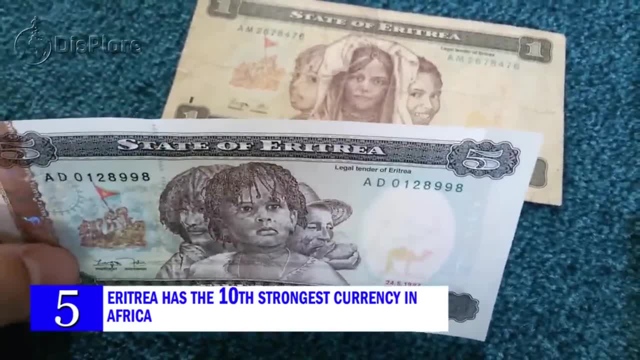 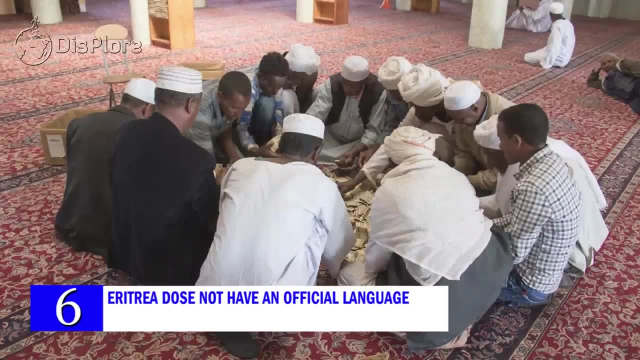 most African countries. The Eritrean Nekfa is currently ranked as the 10th strongest currency in Africa. Number 6: Eritrea does not have an official language. Number 6: Eritrea does not have an official language. 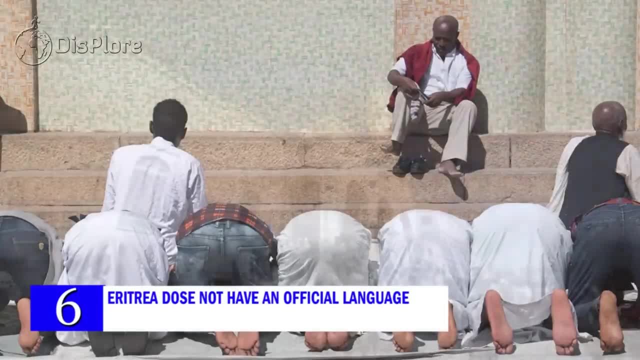 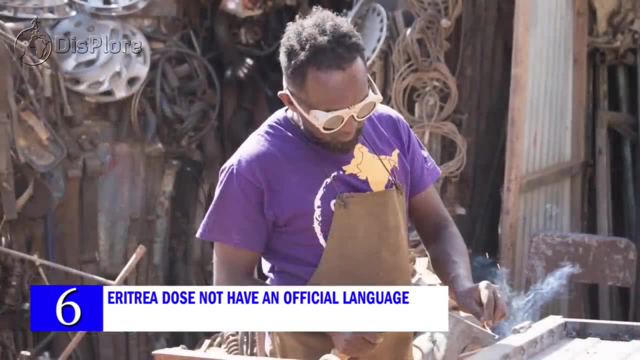 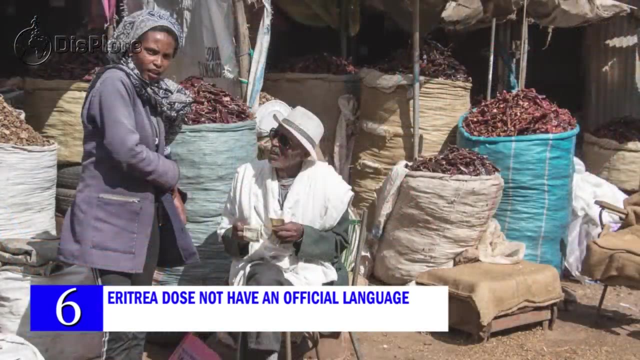 Eritrea is a multilingual country. The nation has no official language. as the constitution establishes the equality of all Eritrean languages, Tigrinya serves as a de facto language of national identity, with about 2,540,000 total speakers of a population of about 5,254,000 in 2006.. 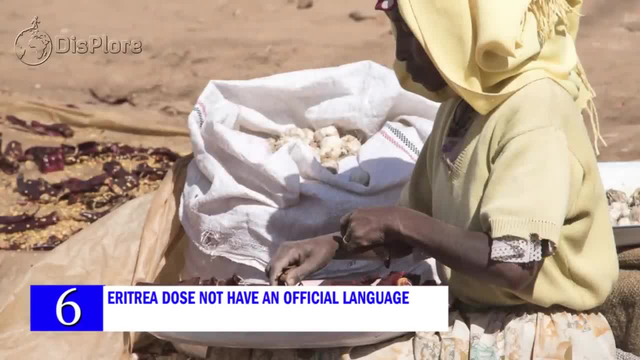 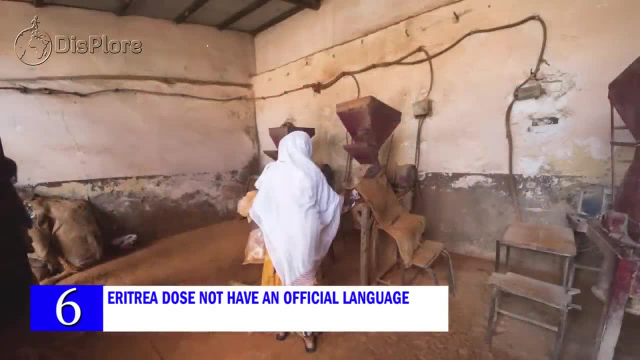 It is the most widely spoken language, particularly in the southern and central parts of Eritrea. Number 8, Tigrinya, is the only language that has a language. nation languages include Afa, Arabic, Beja, Bilen, Kunama, Nara, Saho and Tigre, Tigrinya and. 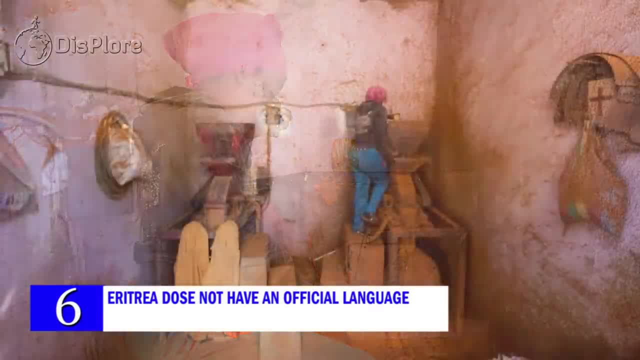 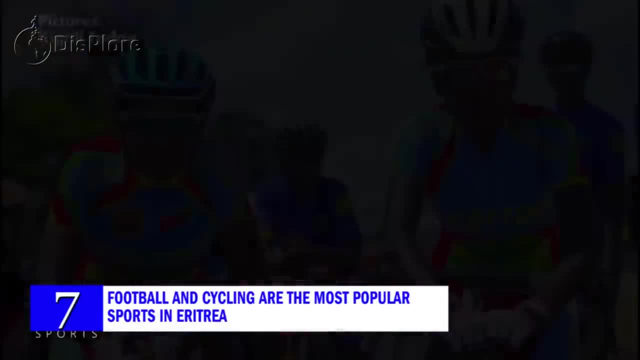 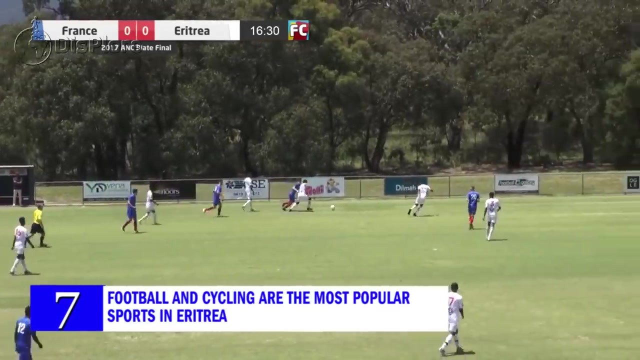 English serve as de facto working languages, with the latter used in university education and many technical fields. Number 7. Football and cycling are the most popular sports in Eritrea. When it comes to football, Eritrea is less popular in that domain, Football and cycling. 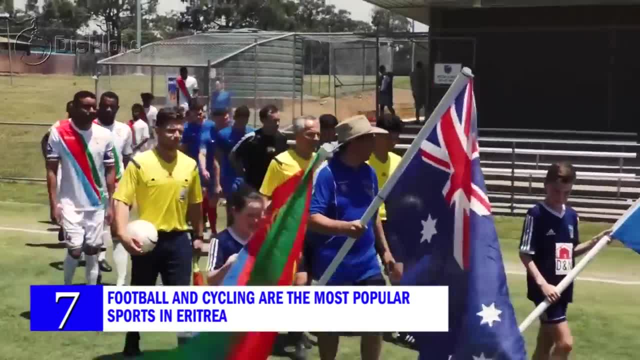 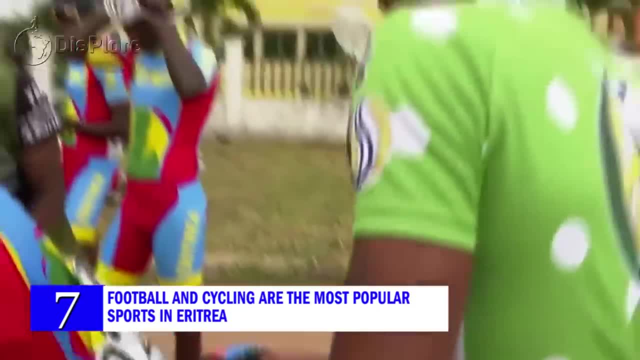 are the most popular sports in Eritrea. In recent years, Eritrean athletes have also seen increasing success in the international scene. Zesene Tadese, an Eritrean athlete, formerly held the world record in the half marathon. The Eritrean national cycling team. 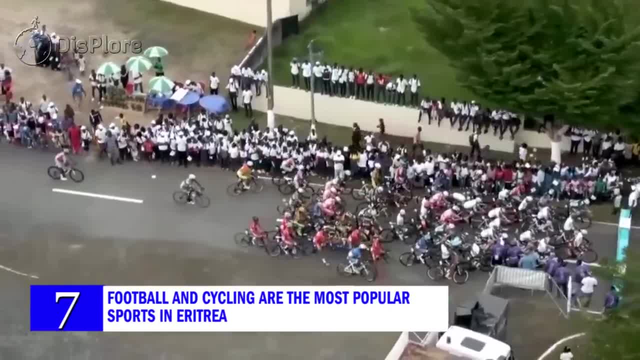 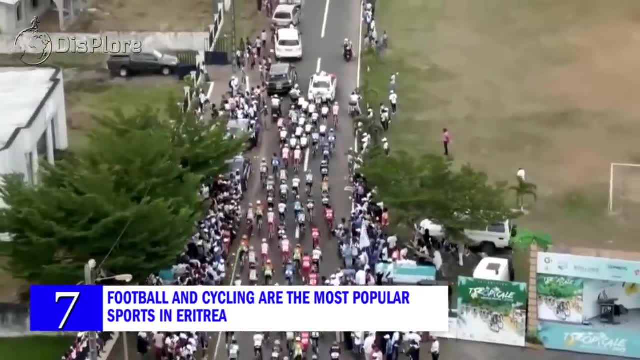 has experienced a lot of success, winning the Continental Cycling Championship several years in a row. The Eritrean national cycling team of both men and women are ranked first on the continent. In 2013,, the women's team won the gold medal in the 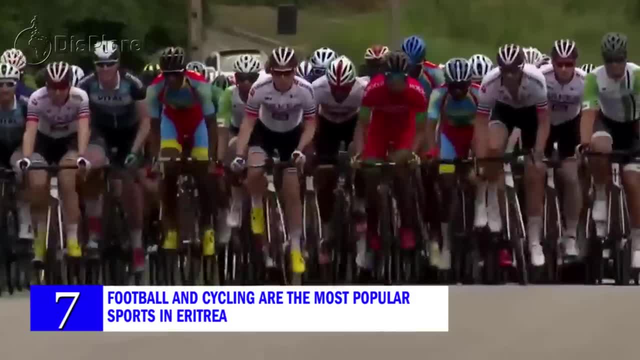 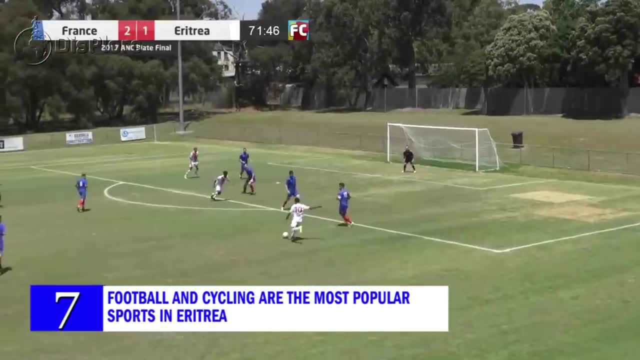 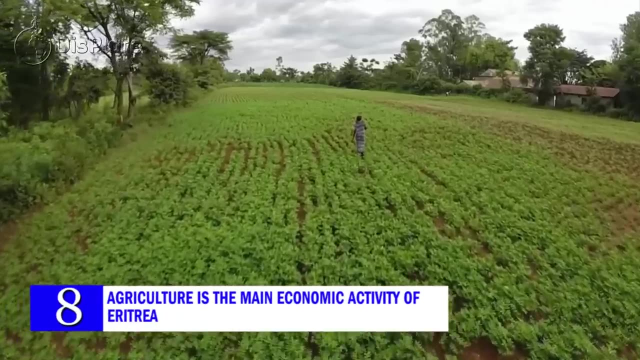 African Continental Championship. for the first time, Six Eritrean riders have been signed to international cycling teams. When it comes to football, Eritrea has never won the African Nations Cup. neither has it ever participated in the World Cup Number 8.. Agriculture is the main economic activity in Eritrea. 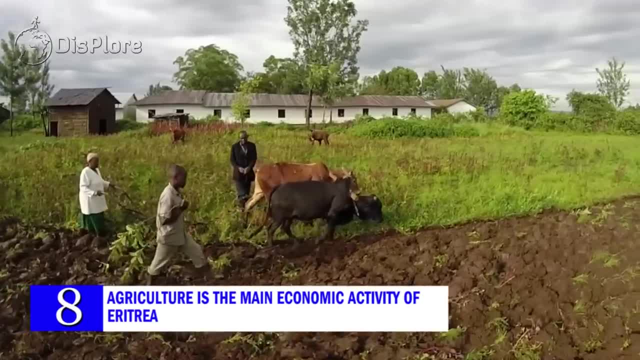 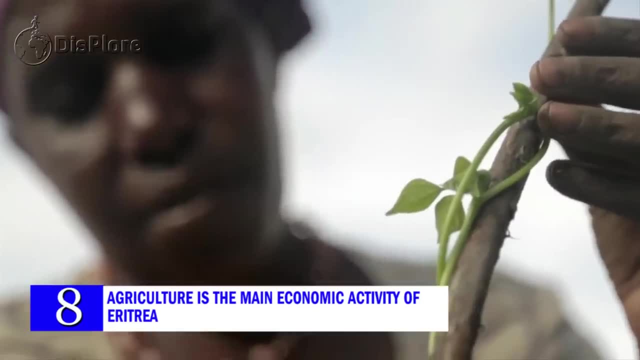 Just like most African countries, the main economic activity in Eritrea is agriculture. About 80% of the Eritrean workforce are employed in agriculture. Eritrea's main agricultural products include sorghum, millet, barley, wheat, legumes, vegetables. 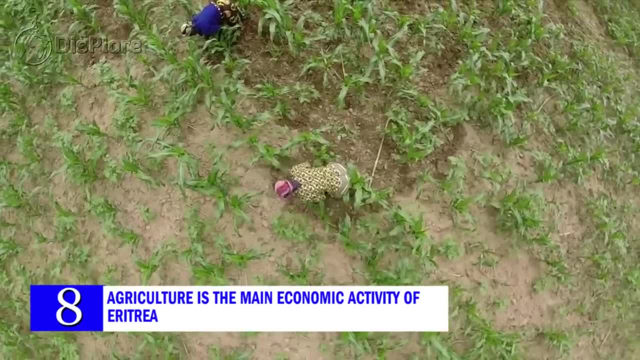 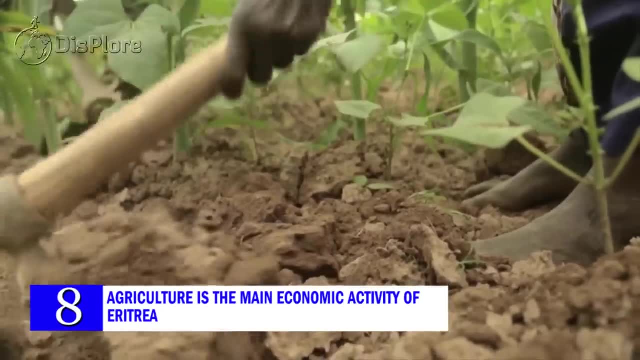 and fruit. The economy of Eritrea has experienced considerable growth in recent years, indicated by an improvement in GDP in October 2012 of 7.5 over 2011.. A big reason for the recent growth of the Eritrean economy is the commencement of full 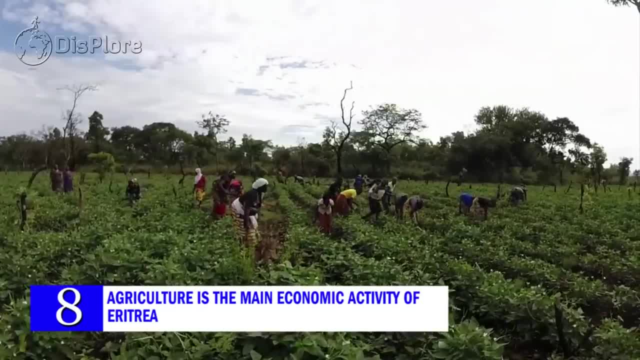 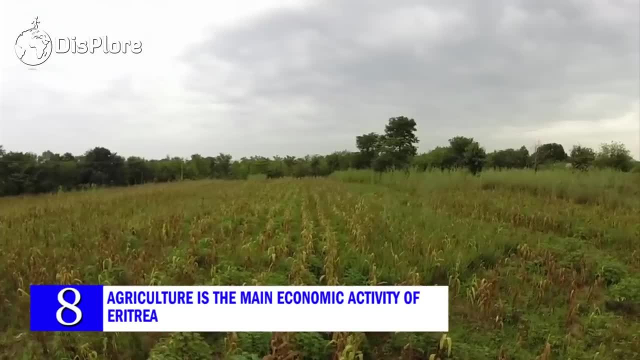 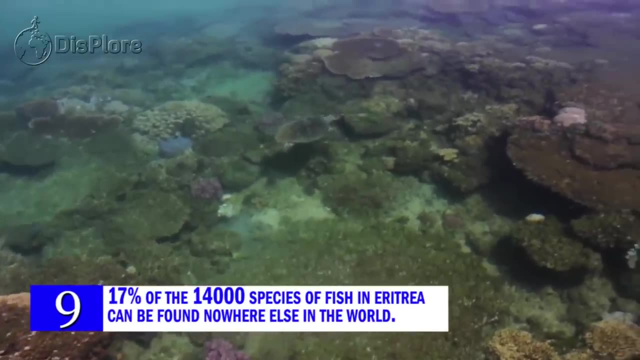 operations in the gold and silver bishop mine and the production of cement from the cement factory in Masawa. The GDP of Eritrea currently stands at $7.7 billion. Number 9.. About 17% of the 14,000 species of fish in Eritrea can be found nowhere else. 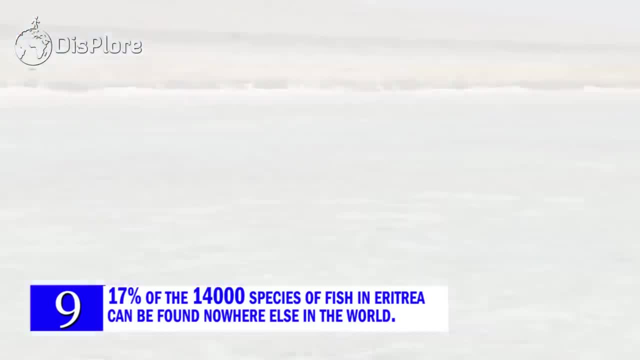 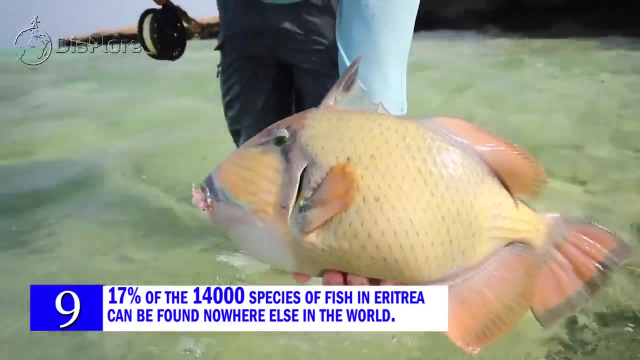 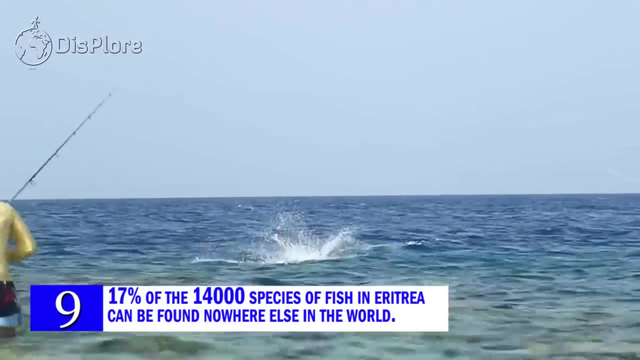 in the world. Having a long Red Sea coastline with warm waters, Eritrea is an attraction zone for rare species of fish. The bulk of Eritrea's fishing zones still hold unexploited potential. Fishing remains a great sporting activity, especially for tourists. You only need to hire a fishing. 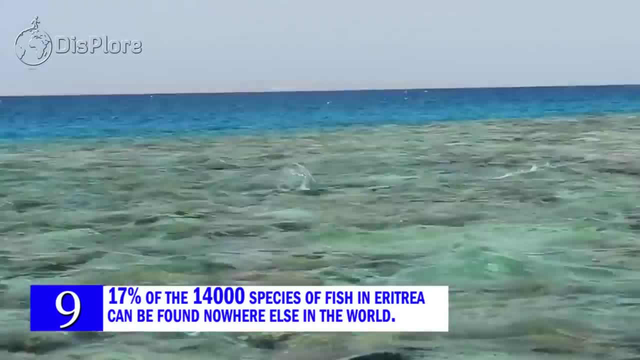 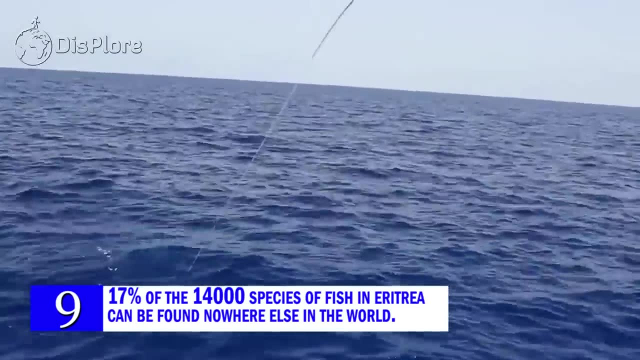 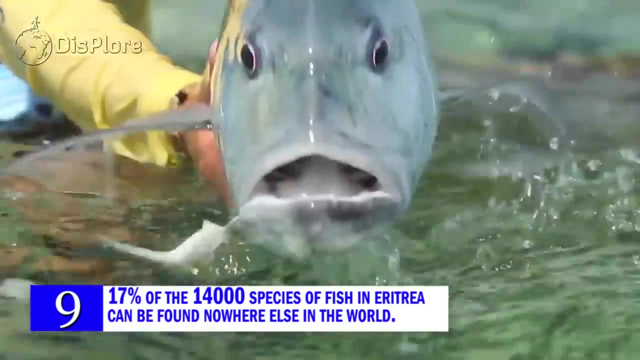 boat and enjoy your activities. The most common endemic marine fish include deepwater dragonet, gobbyoos fish, snailfish, towelfish and stargazer fish, and there are other modernudent assertions about eerythrea as they get bigger by the year 2020.. 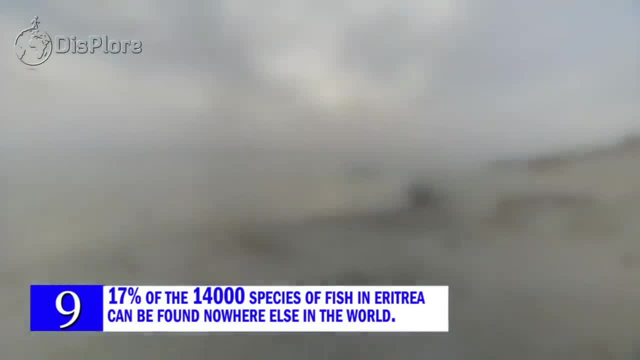 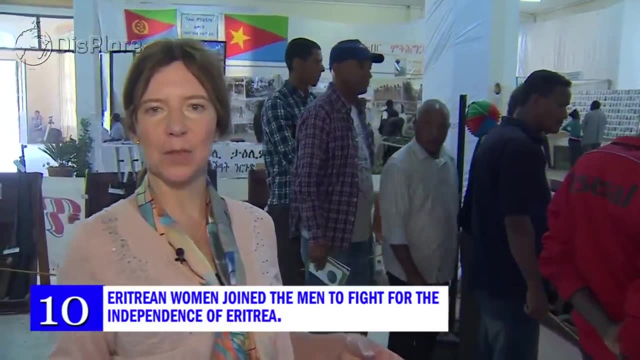 7.0% of the calculatedlette of eerythrea. terrifying, ejecting the inmate with nature's 时候, andREAM is once again zero, Number 10. Eritrean women joined the meant to fight for the independence of Irytyria. 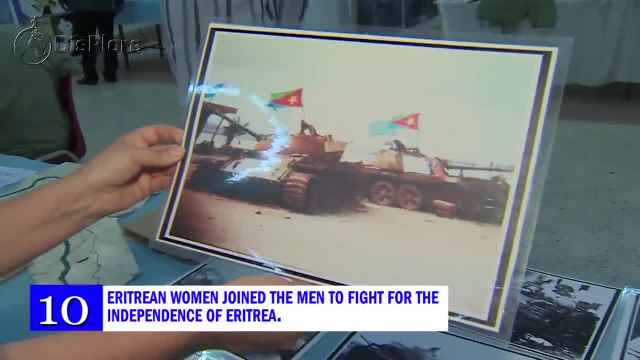 Ten of them made it to the top, while many lost their lives. Whatever their role has been, long Eritrean women picked up arms to help their counterparts fight off the Italians and later the Ethiopians. This is mainly due to the 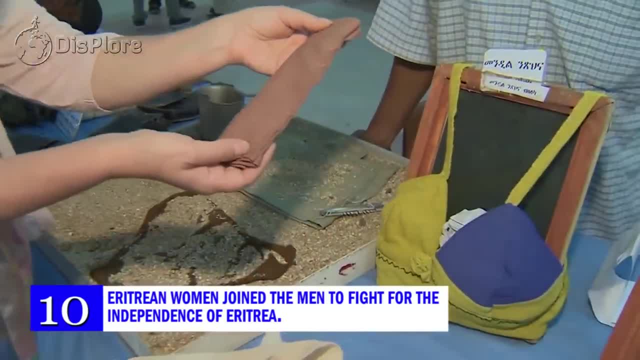 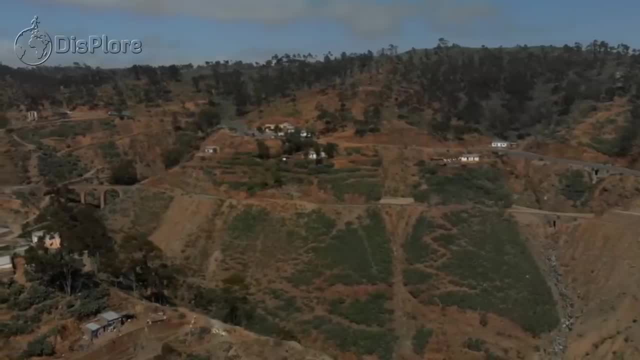 fact that the Eritrean population is small and yet has been engaged in so many wars where hundreds of thousands of men lose their lives. There you have it, Displorers. those were some of the lesser-known facts about Eritrea. you. 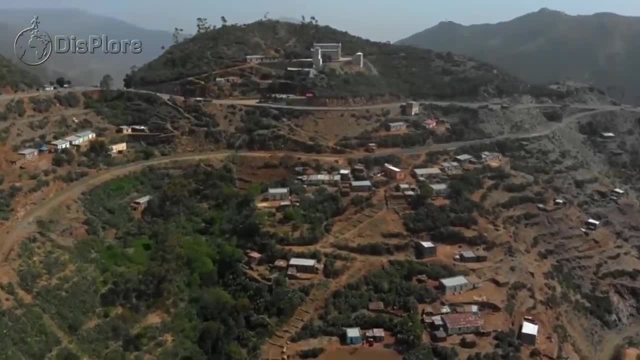 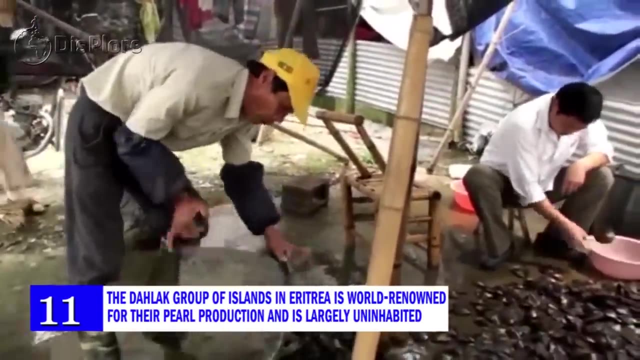 probably didn't know. As a compensation for sticking till the end of this video, here's an extra bonus, fact Number 11. The Dalak group of islands in Eritrea is world-renowned for their pearl production and is largely uninhabited. 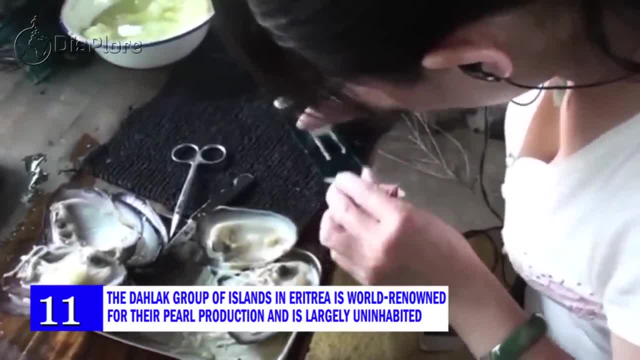 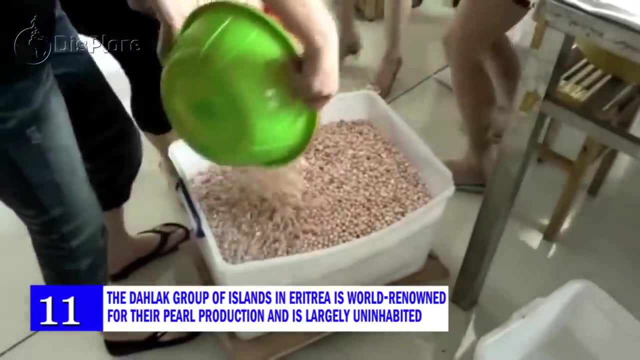 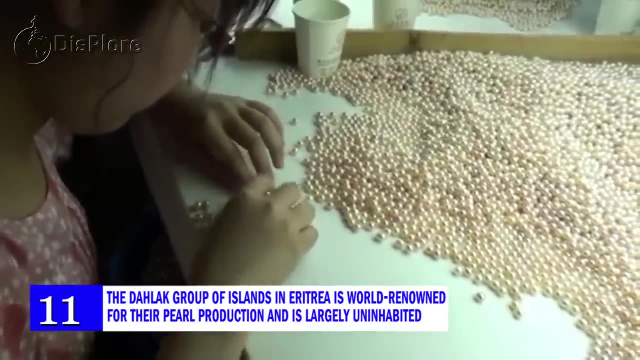 Pearl is treasured in the traditional African society. It was used as a measure of value and a medium of exchange before modern forms of money came in. The Dalak group has kept the tradition of pearl production, though it is no longer used as a medium of exchange. The Dalak archipelago has great tourist. 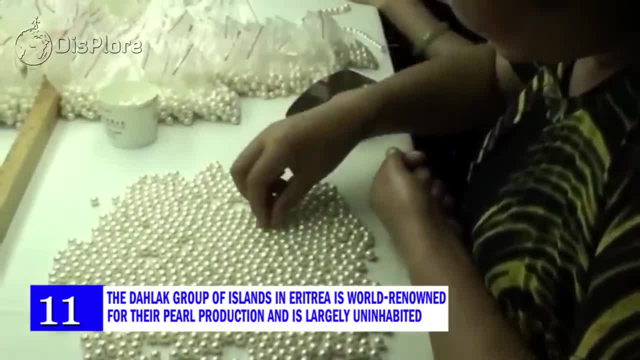 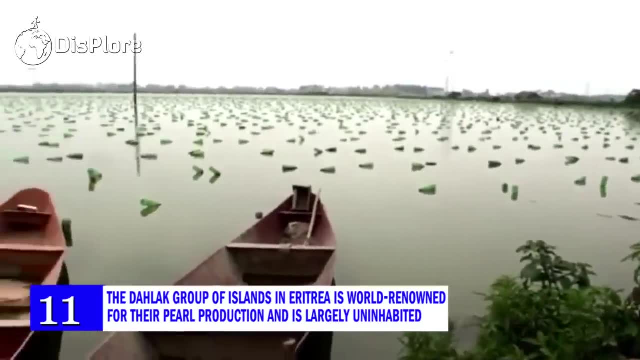 attractions. It is a great place to go scuba diving, pearl fishing and yacht cruising. On the uninhabited side of the islands, you'll find plenty of mangrove trees and salt bushes. There is also a large population of nested birds, coral reefs and 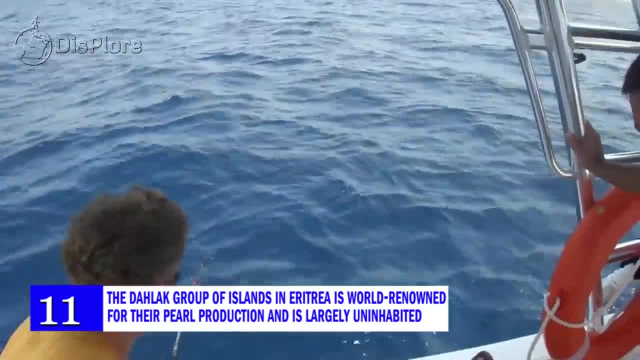 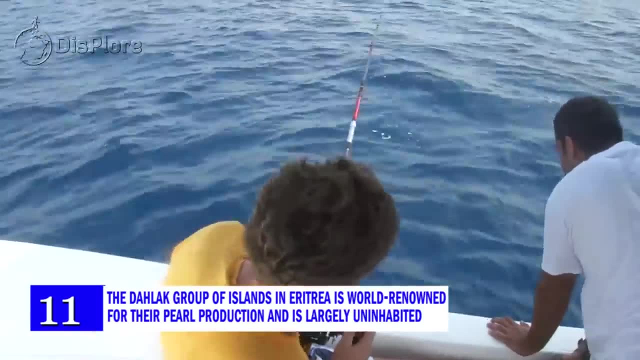 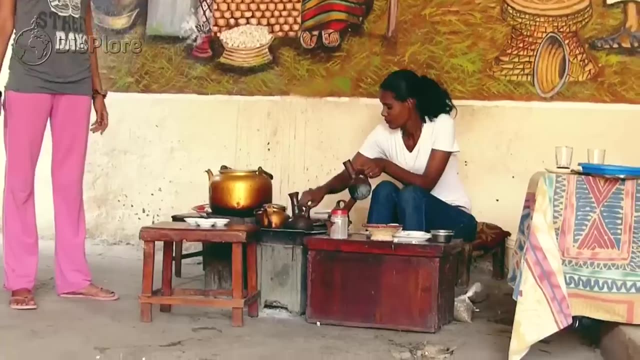 submerged shoals, Plenty of spectacular marine wildlife also exists. These include sharks, hermits, crabs, dolphins, dugongs, shellfish and turtles, amongst many other varieties of marine species. We hope you learned a thing or two from this video, If you know some interesting facts about. 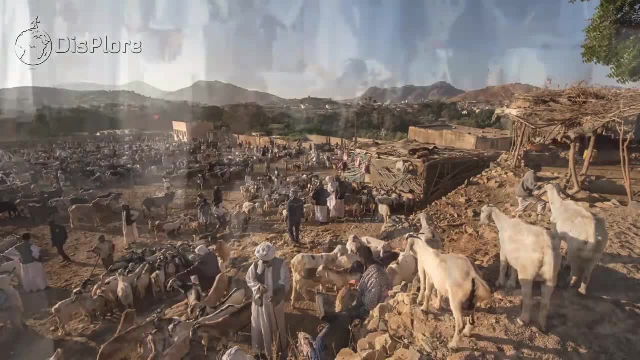 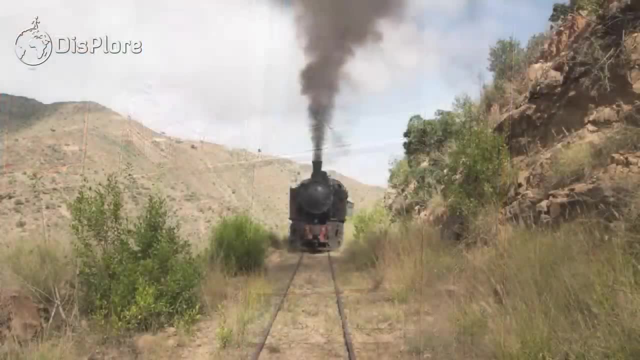 Eritrea that have not been mentioned in this video. please do well to drop it in the comment section below and the best comment will be pinned. Thanks for watching this video. If you did enjoy the video, please give it a thumbs up and do. 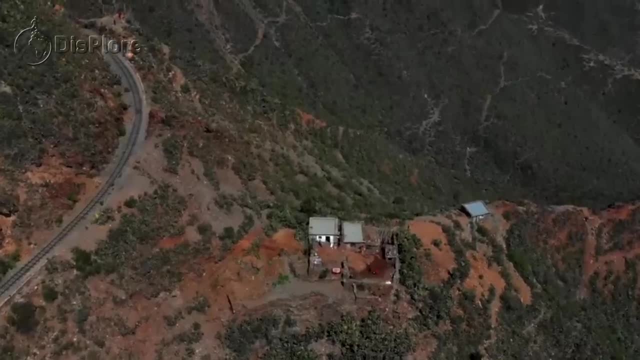 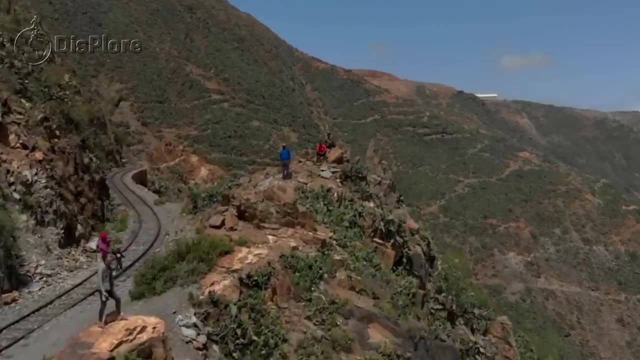 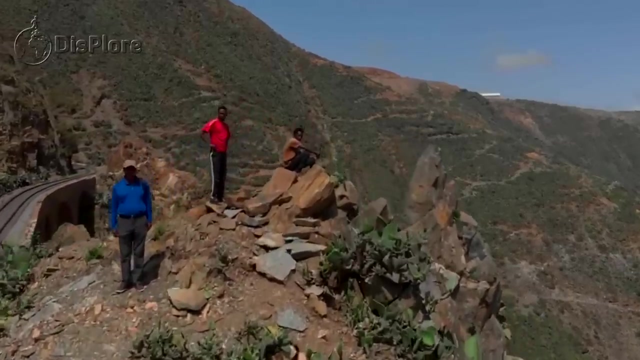 not forget to subscribe and share with your friends. I'll see you in the next video.